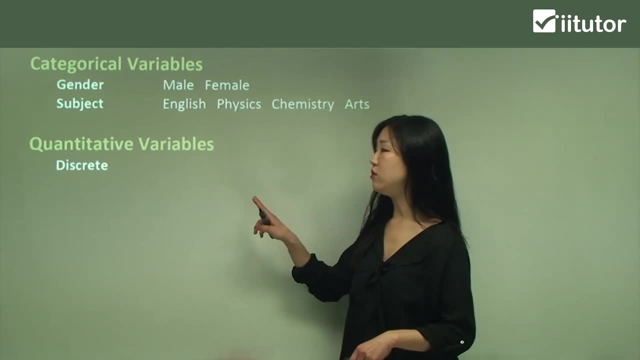 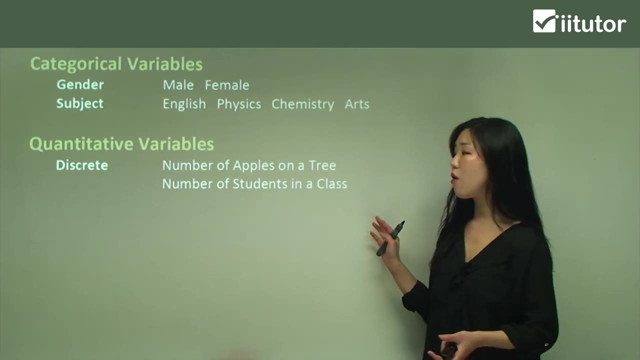 discrete variables. So quantitative variables are discrete, which is, for example, number of apples on a tree or number of students in a class. So as you can see in the examples here, you can kind of see that discrete variables, so quantitative, discrete variables. 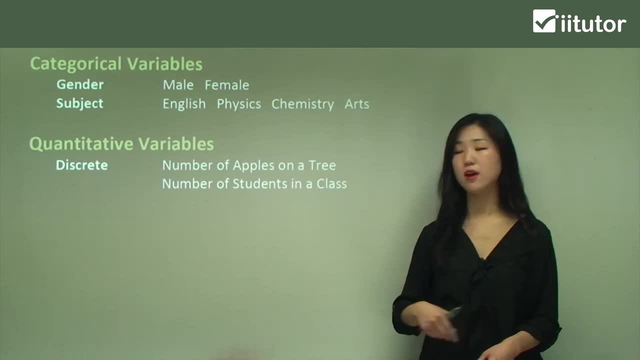 are countable. Okay, so we can count the number of apples on a tree, We can count the number of students in a class, right? So that's kind of like discrete quantitative variables And continuous. so the second one is continuous, which is, for example, weight of a person. We can't count the 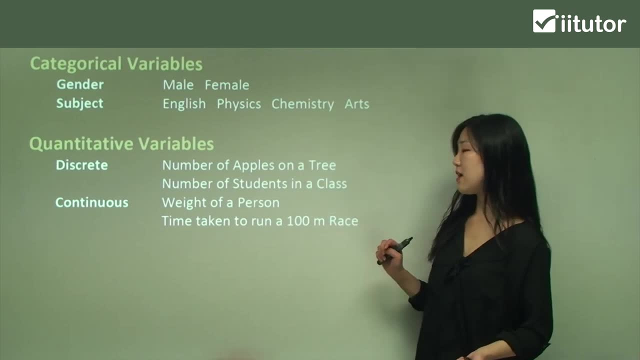 weight of a person. right, It's like a measurement or time taken to run a 100 meter race. So we can't actually count the time right. It doesn't make sense. So those kind of ones, we call it continuous. 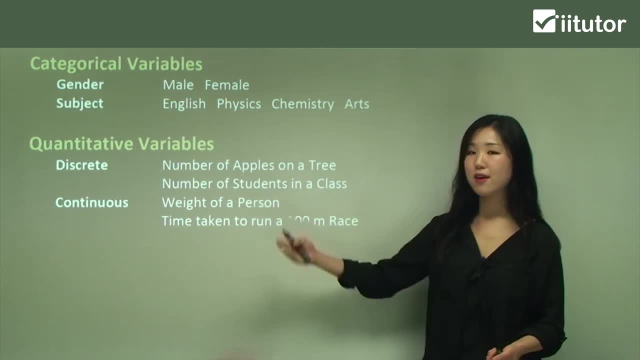 Make sense, guys. So discrete and continuous are two subcategories in quantitative variables. So quantitative is a little bit more extensive because it goes into the two branches. Okay, guys. so remember the two, categorical and quantitative, and remember that quantitative has two separate. 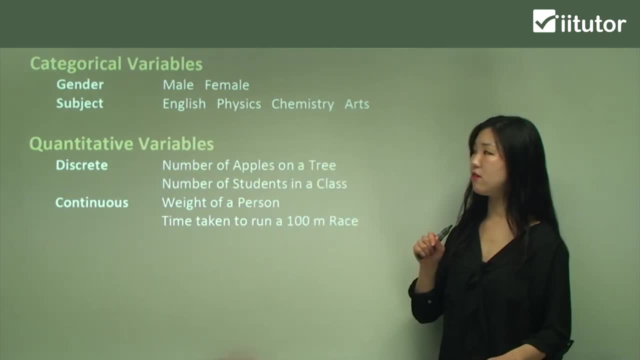 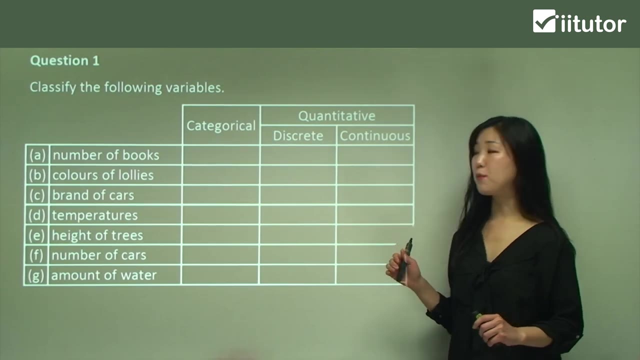 branches that we can classify it into And we're going to try to classify variables now. So question one: it says: classify the following variables. So, as I put here, I've distinguished it into categorical or quantitative. But as I said, quantitative can have, can either be discrete. 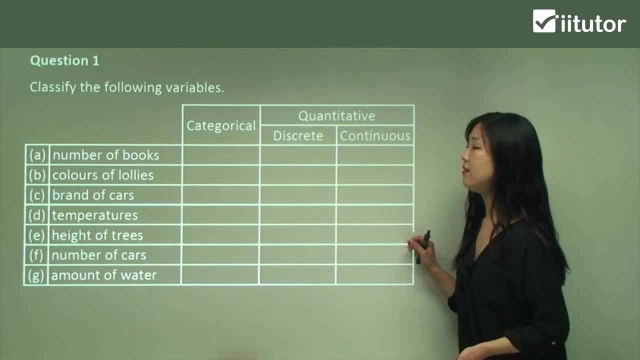 or continuous, so I've separated those two as well. So you're going to help me do this. Let's do A number of books. Now. number of books is a quantity, isn't it? So we're going to be quantitative. 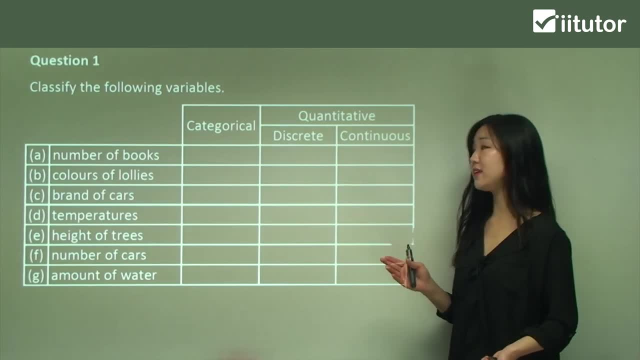 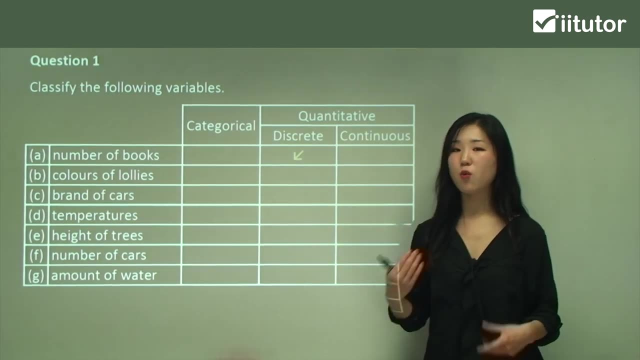 But can we count the number of books? Definitely. So it must be discrete. If it's countable, it's discrete. Now, colors of lollies. Colors of lollies is not a quantity. The color is not defined by a quantity, Rather, it's a category. right Colors can be red, blue, green. We can. 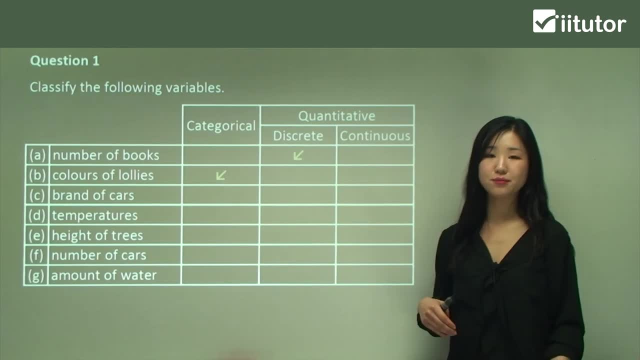 categorize it into color of a lolly, So it's categorical. Now see brand of a car. Yeah, brand of a car like Mitsubishi, Honda or something like that. We can kind of categorize it into a brand, So it's categorical. Temperatures: Now temperatures.